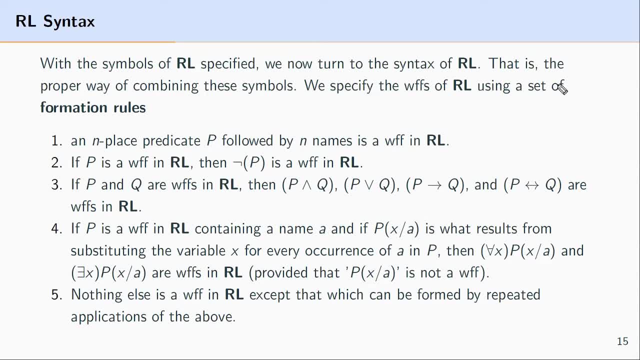 formation rule says that if you have an end place predicate followed by end name, then the result is a well-formed formula. So let's say you have P, and P is a one-place predicate. That means there is sort of one spot after it for a name or term. to kind of go in there Then. 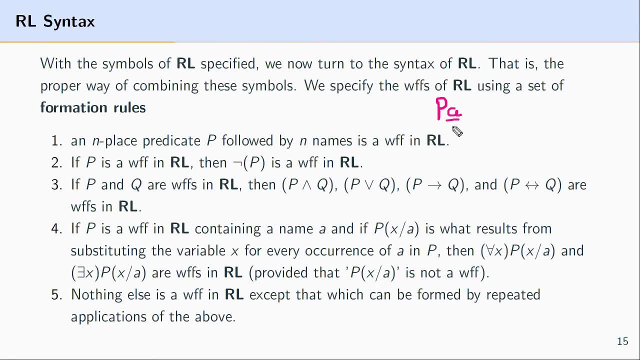 provided there is a single name after it, because, or one name after it, then the result, PA, is a well-formed formula. Now let's say you had a two-place predicate and the two-place predicate was R, And since it's a two-place predicate, there's space for two terms after it. And provided you. 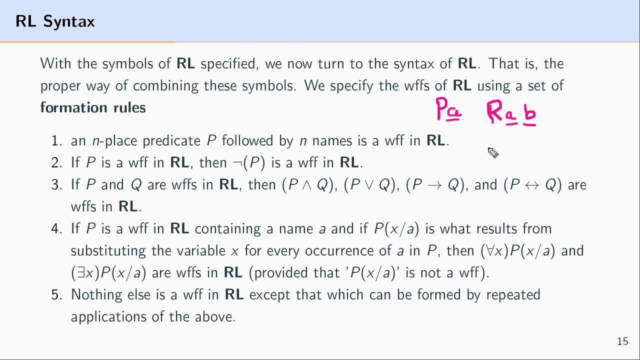 had two names after your two-place predicate, the result would be a well-formed formula. So, with this first rule, what we're looking for is, given some predicate, whether it be P or R or Q, we want to identify the number of places after it. That is what type of predicate it is. And then we want to: 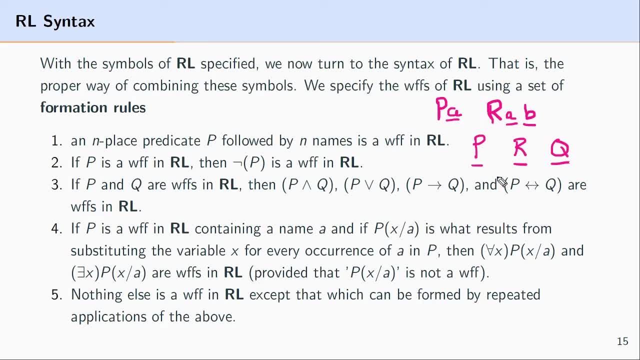 identify the number of places after it. Is it a one-place predicate, two-place predicate, three-place predicate? Once we've identified that, provided it has the appropriate number of names after it, then the result will be a well-formed formula. The next two rules aren't terribly interesting. 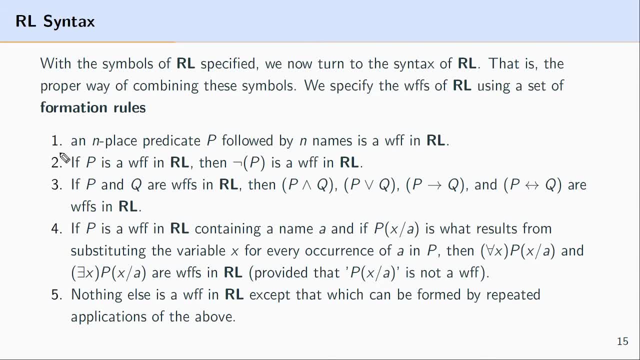 in that they don't introduce anything new from propositional logic. What the second rule states is that if you have a well-formed formula, let's call it P, then the result of negating the entire thing is a well-formed formula. In the case of R, it's a well-formed formula. So if you have a 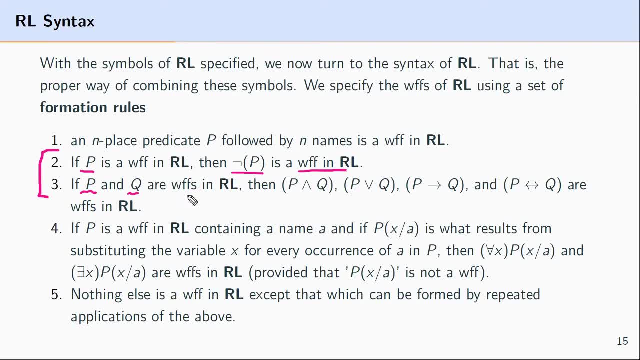 well-formed formula. you can put it together in a conjunction, a disjunction, a conditional or a biconditional, and the result will be a well-formed formula. The next rule states that if you have a well-formed formula, let's say you have P and P is a well-formed formula. 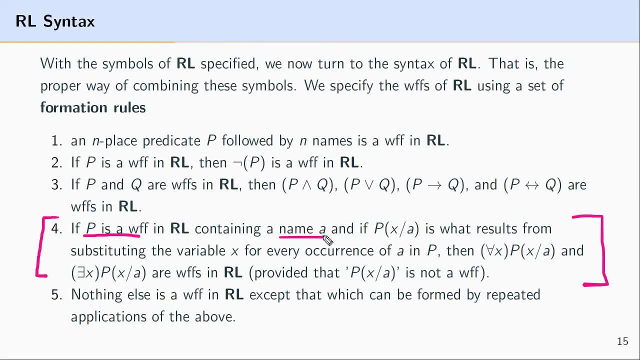 and that formula contains the name A, or any name for that matter, and if P is what results from substituting the variable X for every occurrence of A in P, then the formula AXPXA or EXPXA are well-formed formulas, provided that P is not a. 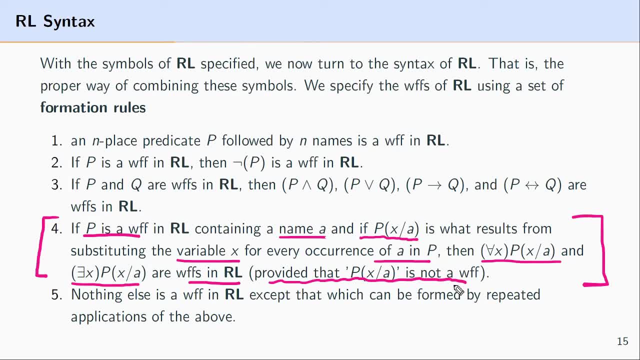 well-formed formula. This rule will require a little bit more specification. It might not be kind of clear what's going on here, So we'll come back to it. What we want to kind of identify now is that here is this rule for forming quantified formulas, for forming well-formed formulas with the quantifier associated with it. 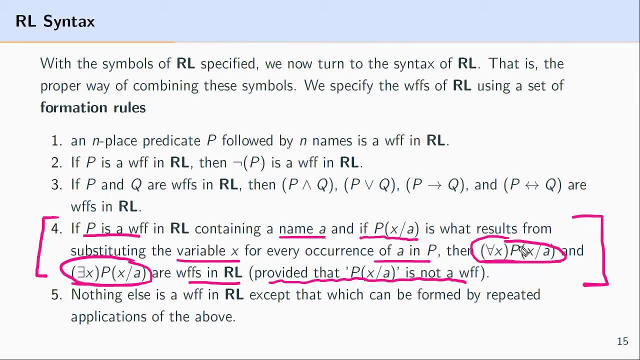 We'll come back to how the whole mechanics of this work in a moment. What this fifth rule states is that nothing else is a well-formed formula in the language of predicate logic, except those formulas that can be formed by reintegrating them into a well-formed formula. So if you have a well-formed 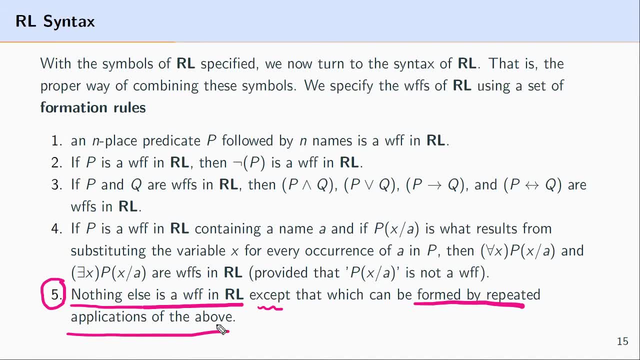 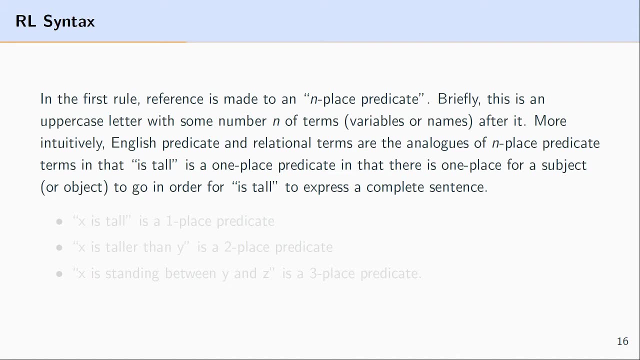 formula, you're going to want to use the repeated applications of the above rules. In other words, the only thing that are well-formed formulas in this language are formulas that can be formed using these four rules right here. So what I'd like to do here is go back to the two new formation. 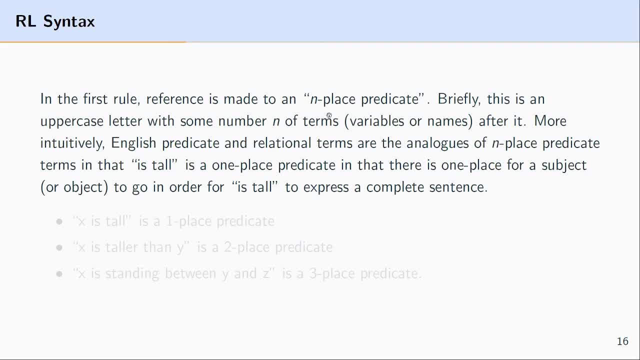 rules. The first rule makes reference to what's known as an end-place predicate. That is, it says that if you have an end-place predicate, let's say P or Q or whatever you want to call it. and you say P or Q or let's say R or S, then provided there are n names after this predicate, then the result 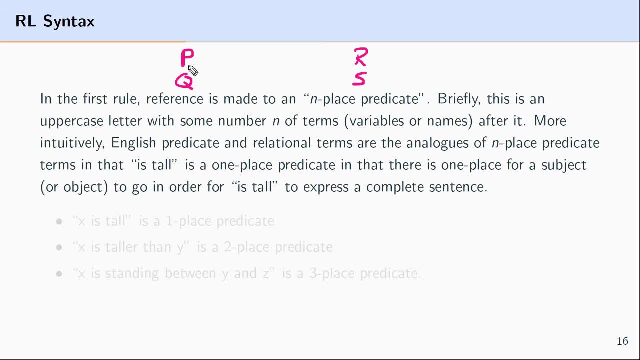 will be a well-formed formula. You can think of end-place predicates in terms of various predicate expressions or relational expressions in English. So, for example, x is tall is a one-place predicate in English And, by the way, this is what we mean is that if you have an end-place predicate, you 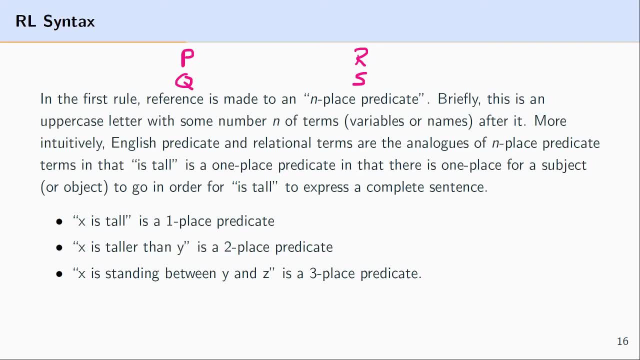 were to put a name in the place of x, you would have a complete sentence. So if you have the one place predicate, x is tall, then if you substitute the name John for x, you'd have the sentence John is tall, And so this is a kind of complete unit here. In the case of is taller than y. what we 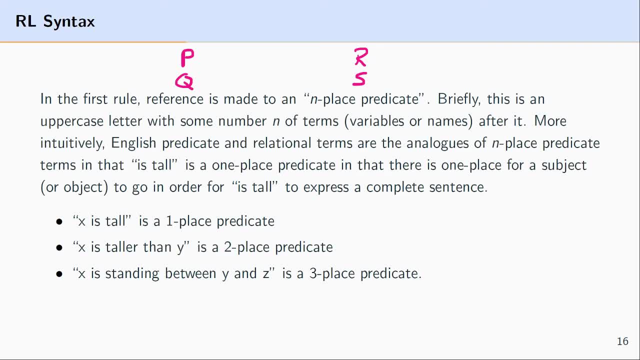 have here is a two-place predicate. There is place, there are two places for names to be slotted in or substituted in. So if you have an end-place predicate you would have a complete sentence. So if we simply said John is taller than and then we kind of stopped, we wouldn't have this. 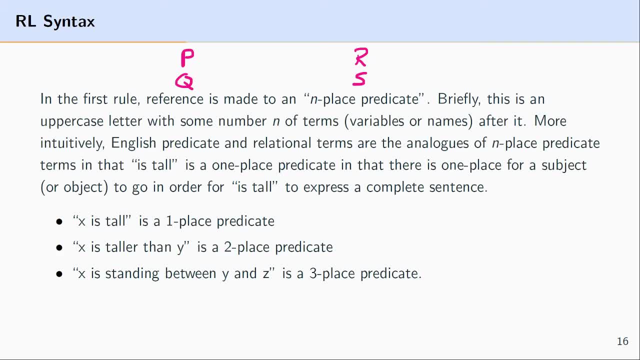 complete unit here. So the two-place predicate is taller than, has two spots or two places for subjects or names to go, And so we could say John is taller than Mary, And again we'd have a complete unit. The same thing would be the case for is standing between x and y. Here we have 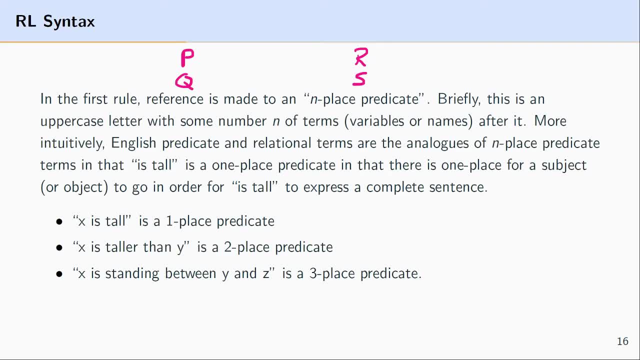 a three-place predicate. There are three spots for names or expressions that designate objects. The same thing is the case for predicate logic. We have various end-place predicate terms and there are the end slots after those end-place predicate terms. So if we have p and we know that p is a, 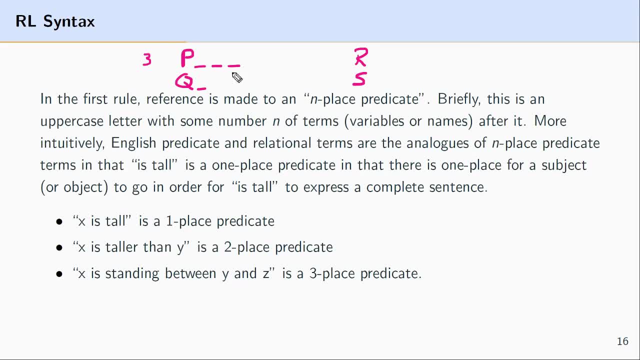 three-place predicate, then we have three spots for names to go. If q is a one-place predicate, then one spot. If r is a two-place predicate, then two spots. And if s is, let's say, a five-place predicate, then we have five spots. What the rule says is that we form a well-formed formula. 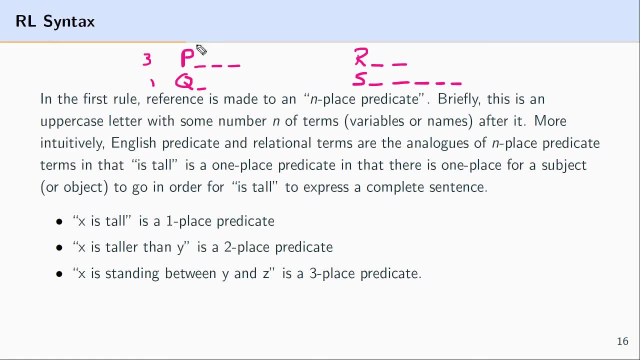 provided once we've identified what type of predicate is- if it's a two- or one- or three-place predicate, provided it has the end terms or end names after that predicate. So if p is a three-place predicate, provided we have three names, then we have a well-formed formula. 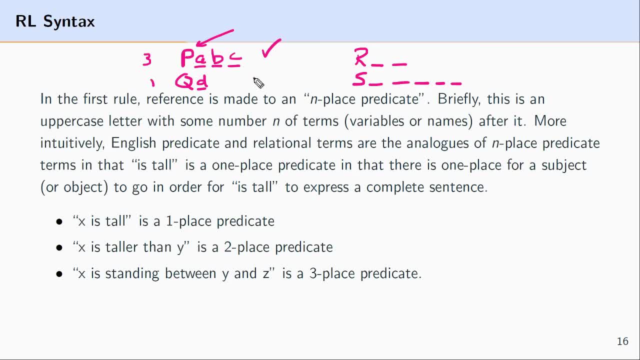 If q is a one-place predicate and we have one name, then qd is a well-formed formula. Now, if r is a two-place predicate and we have only one name, where we have this sort of missing spot here, then at least how the rule is formulated this is not a well-formed formula. 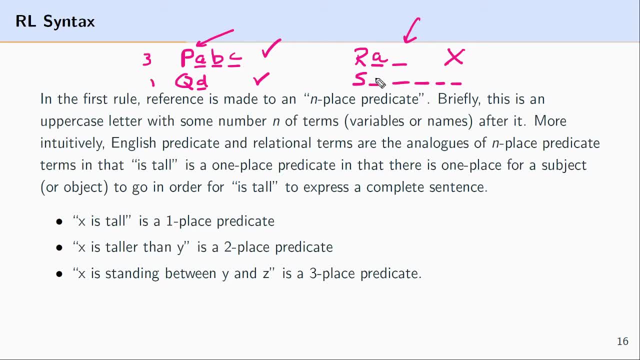 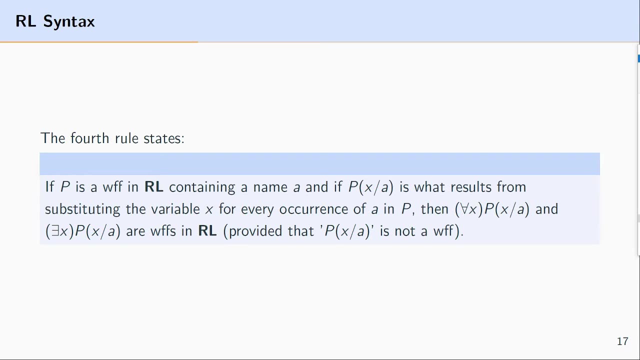 And if s is a five-place predicate and we only have two terms, a and let's say a again- then we don't have five names after The s, and so it is not a well-formed formula. So now I'd like to look at the fourth formation rule, because I think it's the most complicated. 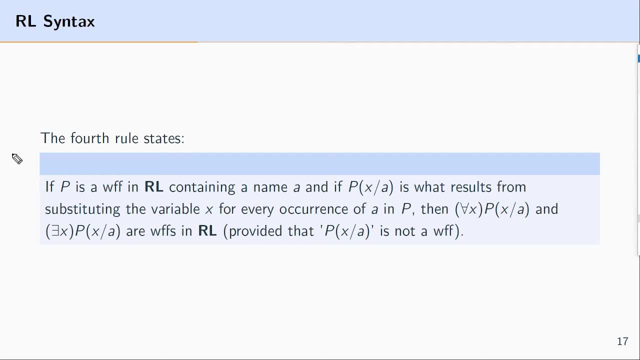 or the one that's most difficult to understand. So I'd like to look at this rule by walking through an example. So the beginning part of the rule states that: suppose that p is a well-formed formula in the language of predicate logic and that formula contains the name a, but it can be any name. 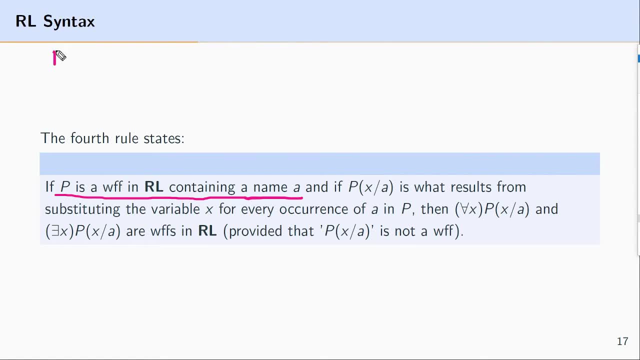 So let's take an example. Let's say we have a one-place predicate. It's a predicate and it's p a. Next, let's suppose that px slash a is what results from substituting the variable x for every occurrence of a and p. 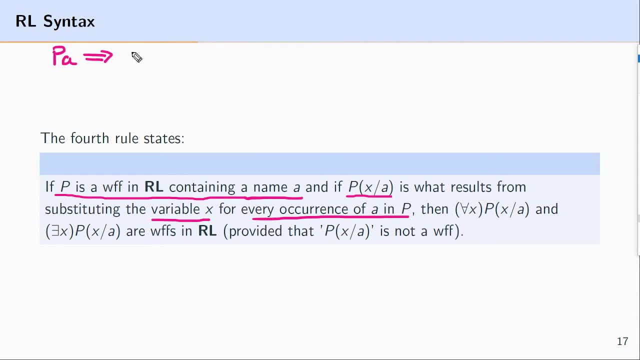 So what we're saying here is: imagine a sort of substitution process where we go about replacing each instance of a with x. So in this particular case, what it would give us is: we're replacing every instance of a with x. It would give us px, and this is not a well-formed formula. 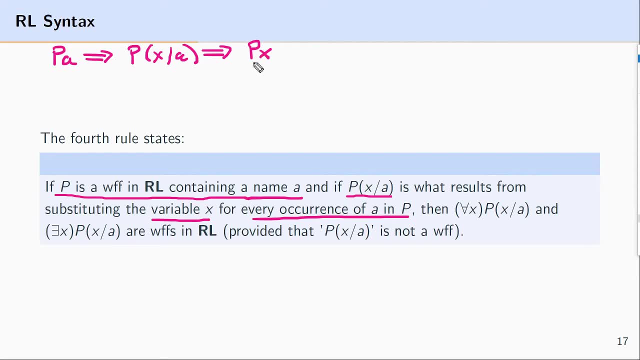 at least is how we've defined it. Then the rule states that we can put a universal quantifier as well as a variable that we used to in the substitution process, in front of the result of this substitution, and the result will be a well-formed formula. 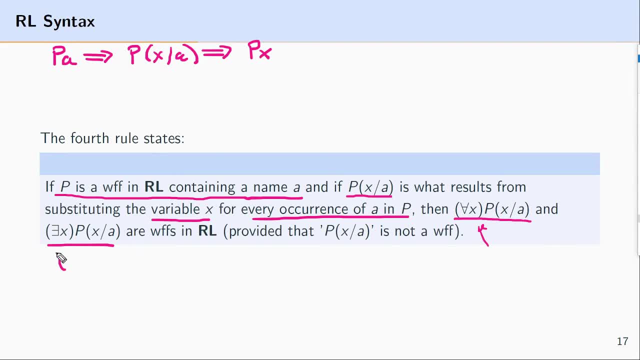 Or we can put an existential quantifier along with the variable x, which is the one that we use to substitute for the names, and the result will be a well-formed formula in the language of predicate logic. So just to look at our particular example here, p is what results from replacing 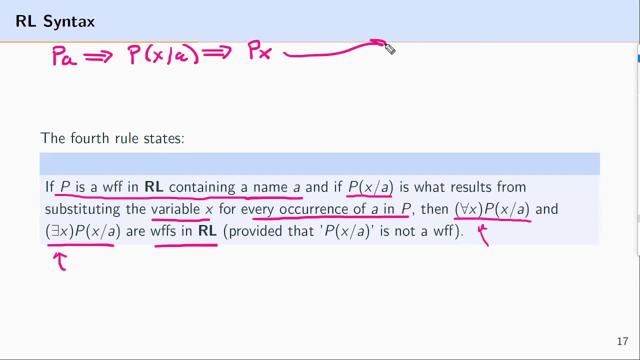 a with x, and so we can take this particular formula and place a universal quantifier along with the variable that we used in the substitution process in front of this formula. so a upside down: ax, px, and the result is a well-formed formula. 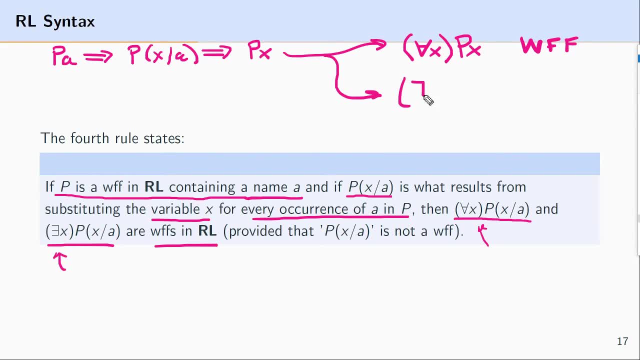 Or we could put the existential quantifier in front of this formula and the result would be a well-formed formula. So this is how you make use of the fourth formation rule to form well-formed formulas that involve the universal quantifier. Let's look at one more example. 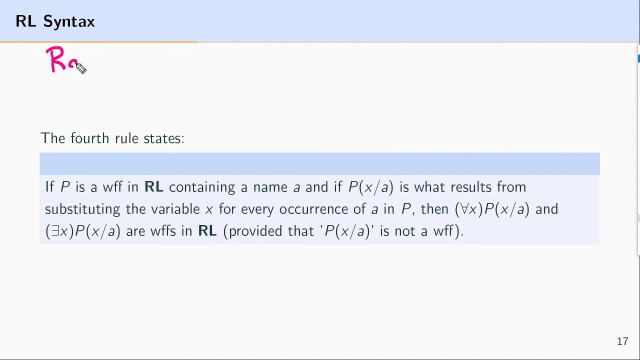 Suppose we have r, a, b and we'll suppose that r is a two-place predicate and since there are two names after r, we have a well-formed formula. So we meet this condition. so if p is a well-formed formula in the language of predicate logic, 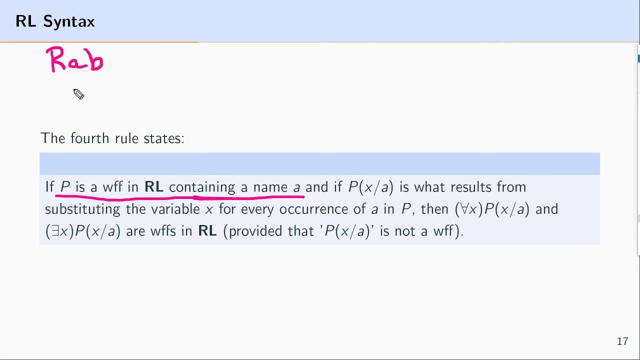 and it contains a name, and so we have this well-formed formula. Now suppose that r y b is what results from replacing each instance of b with the variable y. So this sort of substitution process would give us r a, y. 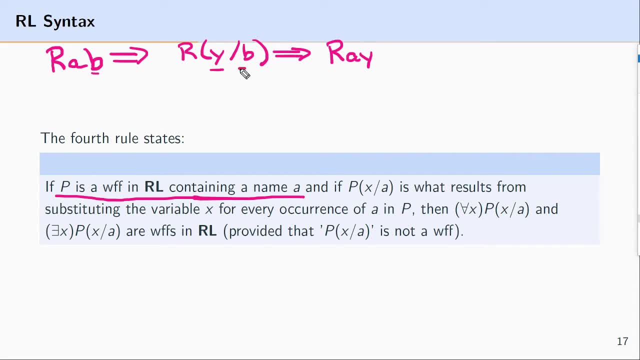 So what we're doing here is replacing each instance of b with a- y. Now, given that we have r a y here, we can place either the universal quantifier in front of it- a y, r a y- and the result will be a well-formed formula, or we could put the existential. 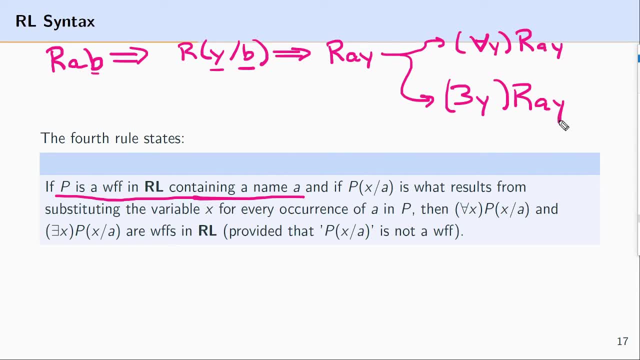 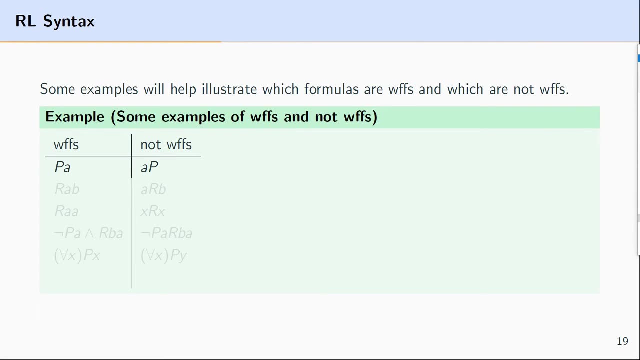 quantifier in front of it- r a, y- and the result would be a well-formed formula. So this is another example how we might make use of this fourth formation rule to form well-formed formulas that involve quantifiers. So it's helpful to finish up this discussion by briefly talking about 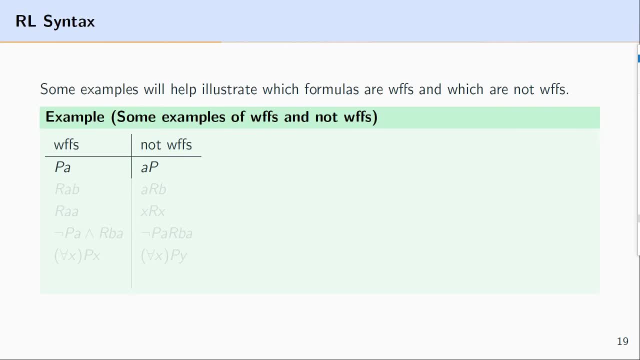 or, briefly, looking at a variety of well-formed formulas, formulas that are well-formed formulas and formulas that are not well-formed formulas. So let's start by looking at p, a p, a assuming p is a one-place predicate- says it's followed by a single name. it's a well-formed formula, The name. 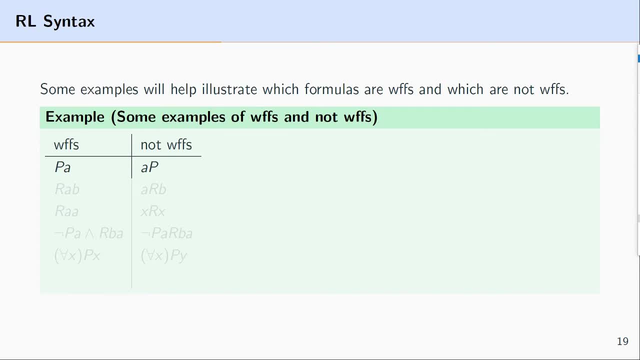 comes to the immediate right rather than the immediate left or above it or below it. In contrast, a p is not a well-formed formula because the name needs to come to the immediate right of the end-place predicate, not to the left or above it, or below it or way out in left field. 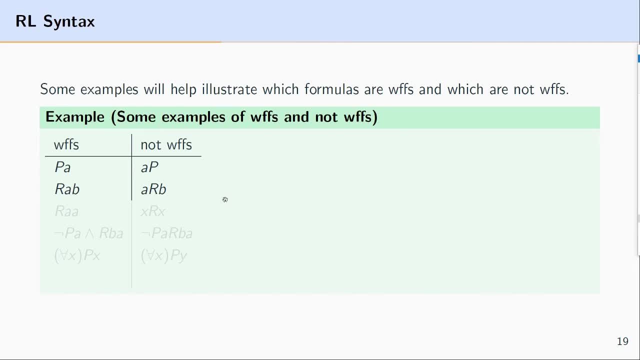 r a b, assuming r is a two-place predicate is a well-formed formula. It's a two-place predicate followed by two names that come to the immediate right. so it's a well-formed formula. a, r, b is. 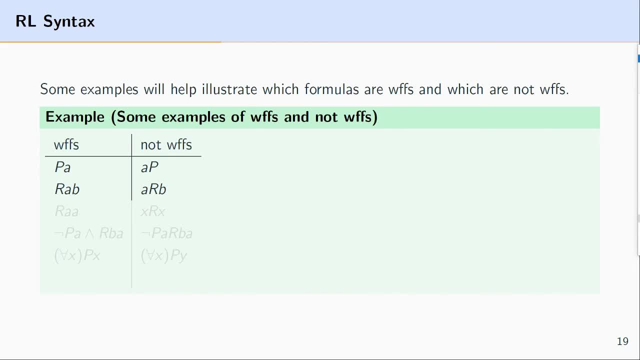 not a well-formed formula because again, the names need to come to the immediate right. It has two names, but they're just not to the immediate right. r, a, a is a two-place predicate, with two names to its immediate right, Even though it's the. 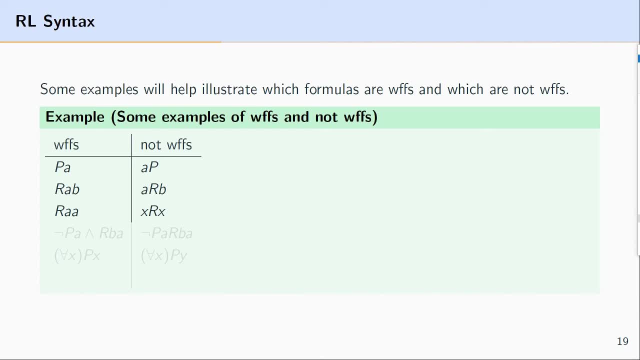 same name. it doesn't disqualify it from being a well-formed formula. It just needs two names to fill the spot. It doesn't matter what names they are. x, r, x is not a well-formed formula one because it doesn't have any names in it and how we formulated the rule in this case. 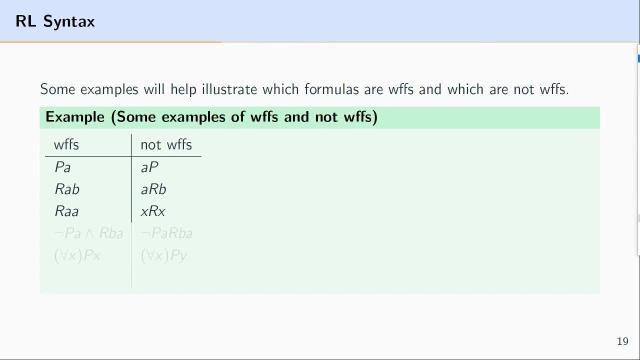 is that there needs to be names following it rather than, let's say, variables, not p a and r, b. a is a well-formed formula. Here we have two well-formed formulas and they're put together using the conjunction rule, whereas not p a, r, b a, even though you 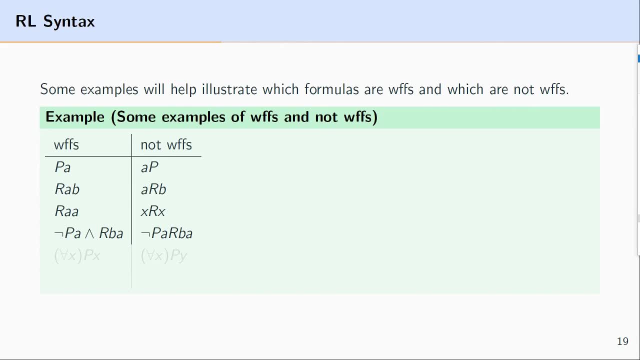 have these and the appropriate number of names. it's not put together using the correct propositional rule. Finally, assuming p is a one-place predicate, we can make use of the formation variables to create this particular formula: ax- px. We already showed an example of how we said. 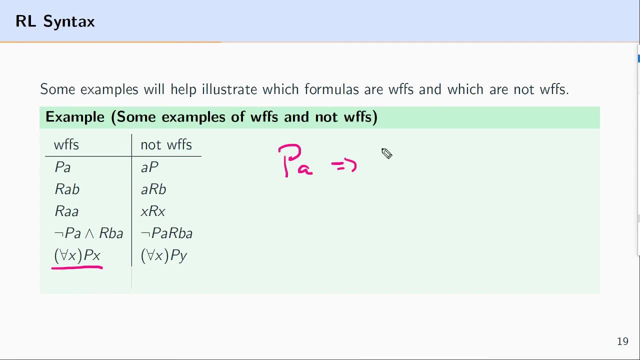 okay, let's say p is a well-formed formula and then we can have this process where we replace a with x, and then we can take what's results from that and put a universal quantifier in front of it, and it would give us a ax px. In contrast, ax py is not a well-formed formula because there's 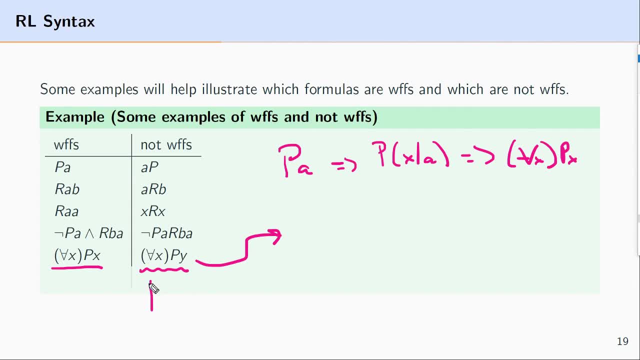 of this fourth formation rule, to have a universal quantifier with a x in front of it where it's quantifying over, or the result is this py. to see this, let's say we start with a pa again. now we want to get this sort of py here. but here we're at a kind of crossroads. we say, well,